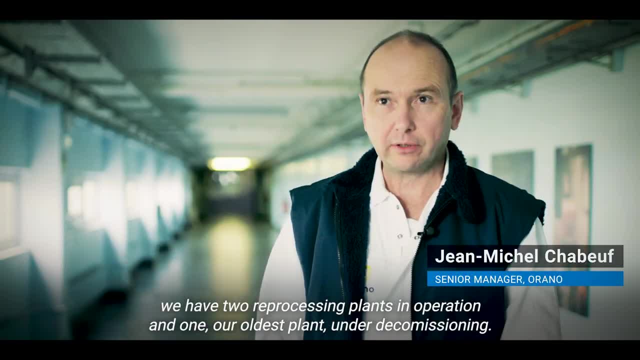 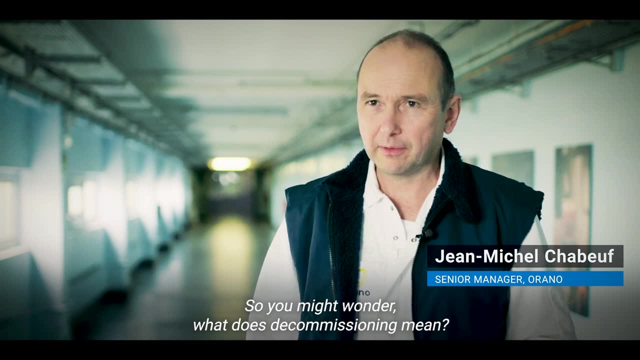 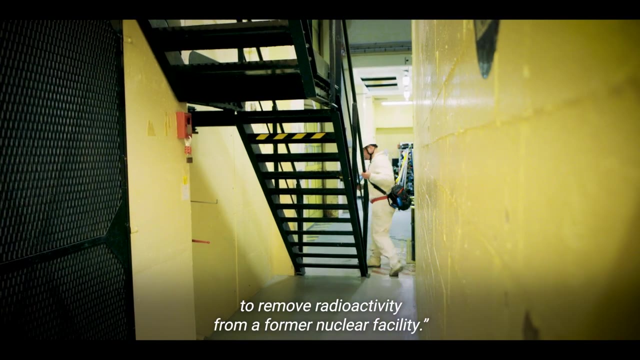 On the site of La Hague, we have two reprocessing plants in operation and one- our oldest plant, under decommissioning. So you might wonder: what does decommissioning mean? Well, decommissioning covers all the activities that are needed to remove radioactivity from. 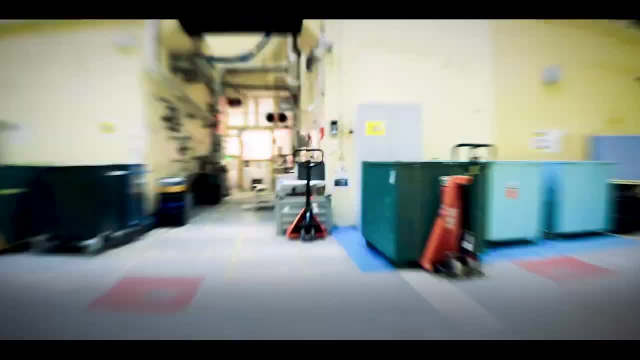 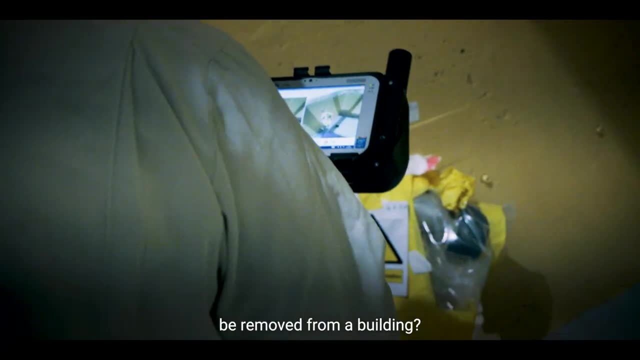 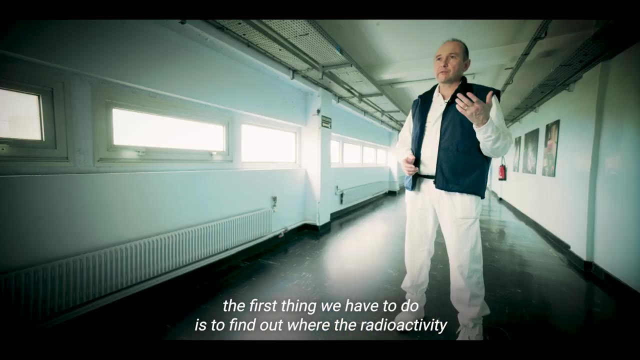 a former nuclear facility. But how exactly can radioactivity be removed from a building? When we receive a facility for decommissioning, the first thing we have to do is to find out where the radioactivity is located, how strong it is and in which form. 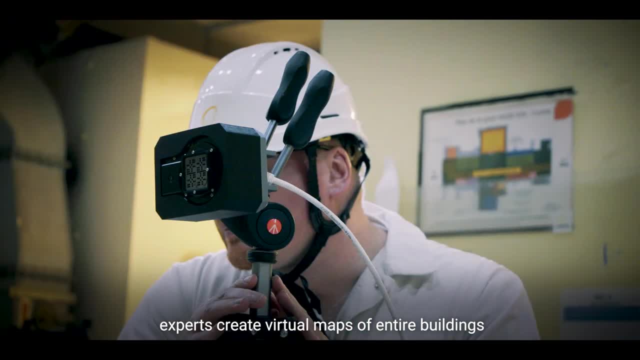 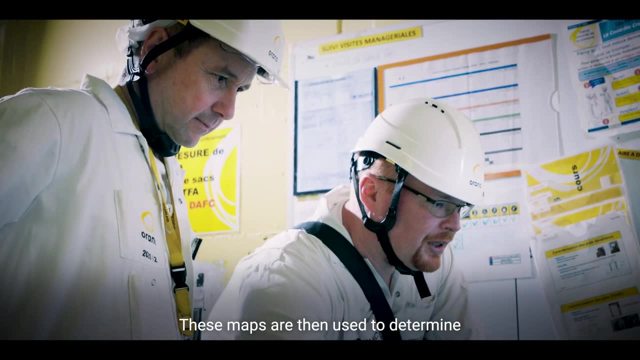 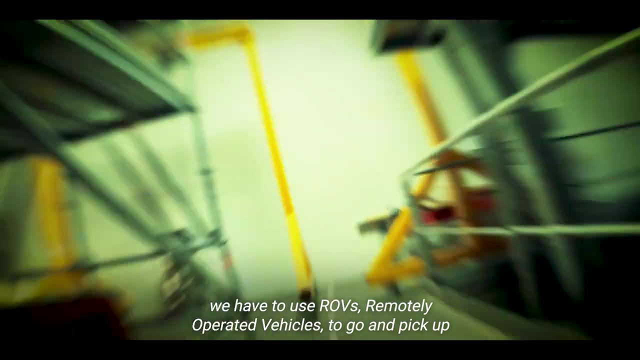 With special equipment, cameras and software experts create virtual maps of entire buildings which show all radioactive areas. These maps are then used to determine how to decontaminate a facility In highly radioactive environments. we have to use ROVs, remotely operated vehicles, to 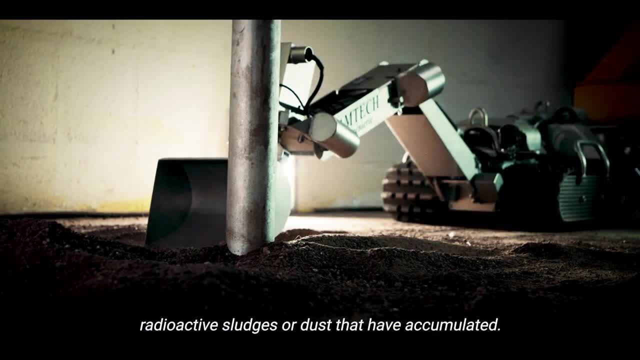 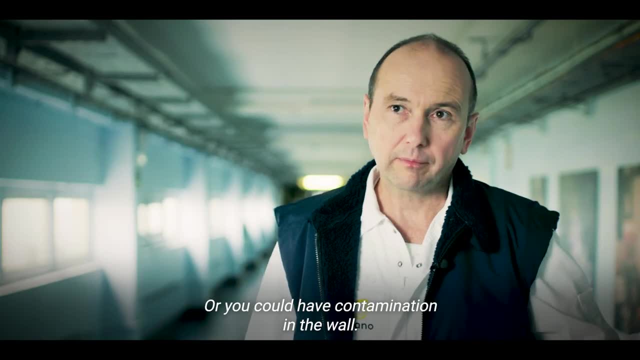 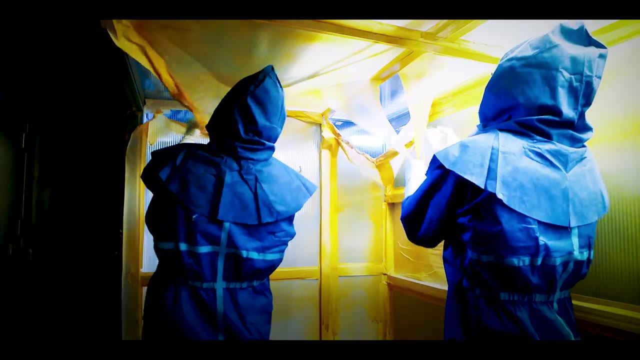 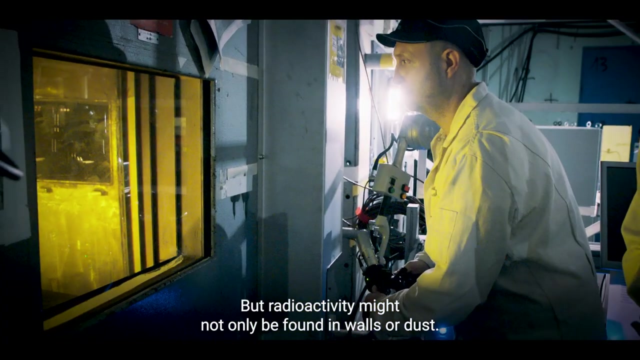 go and pick up radioactive sludges or dust that have accumulated, Or you could have contamination in the wall. In this case we have special resins that we can spray on the wall and then peel to remove the contamination. But radioactivity might not only be found in walls or dust. 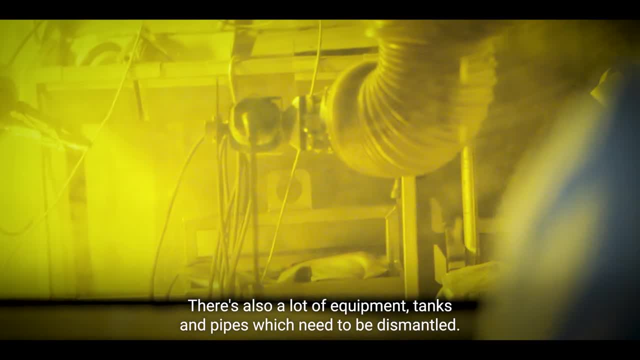 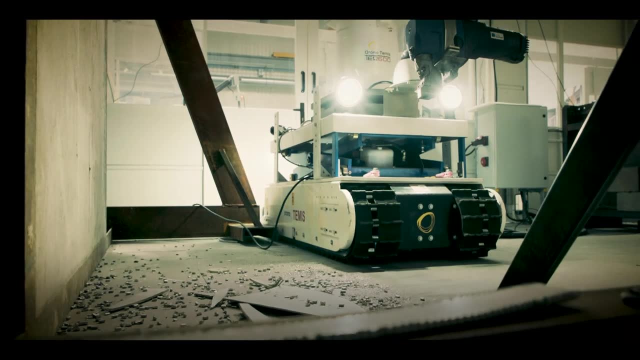 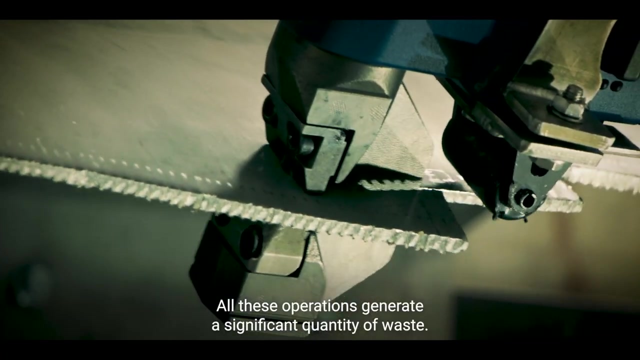 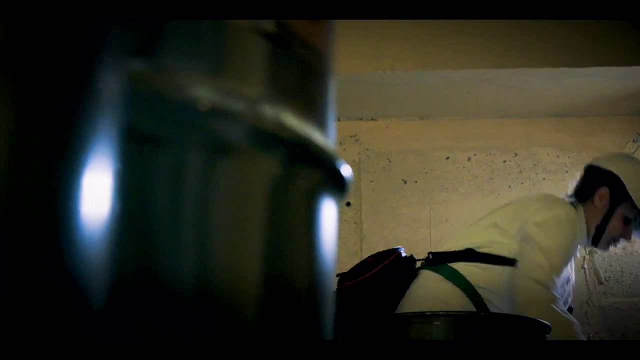 There is also a lot of equipment, tanks and pipes which need to be dismantled In environments that are still too radioactive. robotic systems help out. All these operations generate a significant quantity of waste. The vast majority of this waste is conventional and can be reused and recycled. 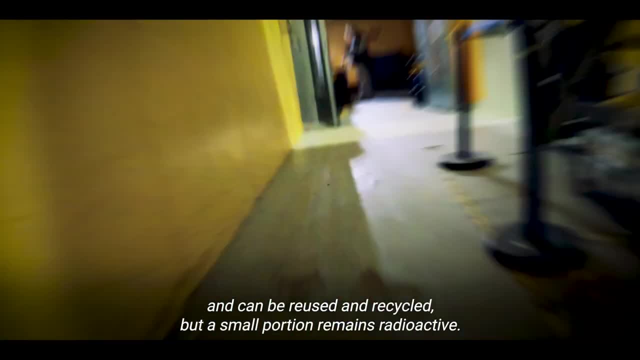 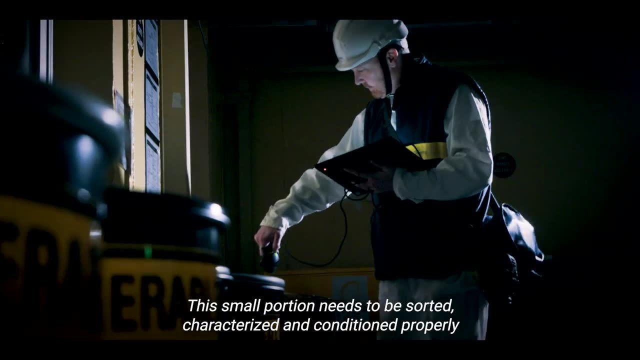 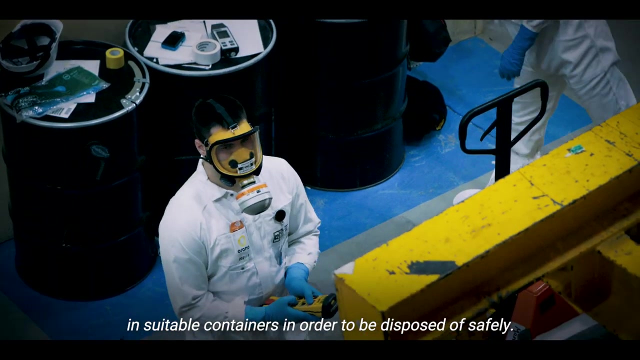 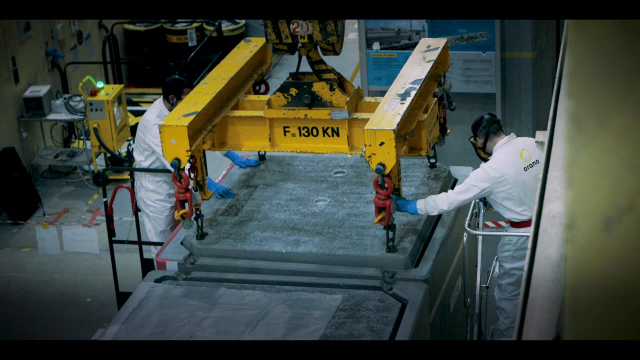 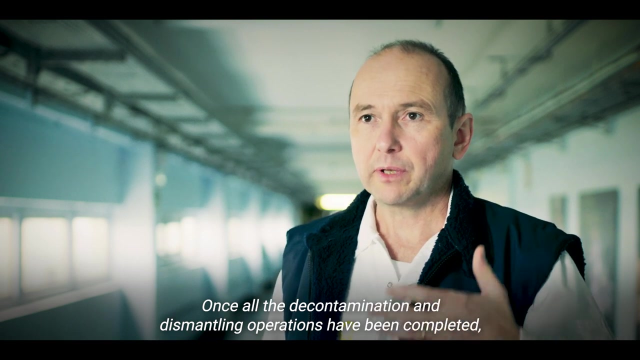 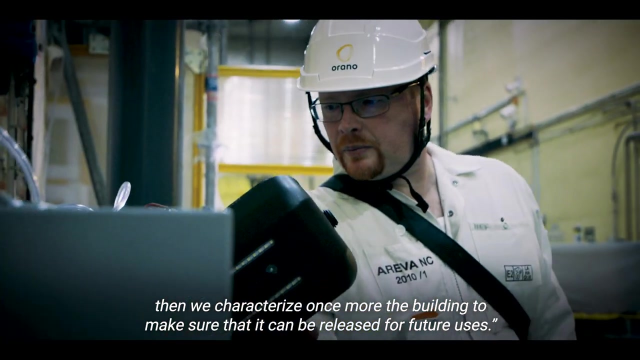 But a small portion remains radioactive. This small portion needs to be sorted, characterised and conditioned properly in suitable containers in order to be disposed of safely. Once all the decontamination and dismantling operations have been completed, then we characterize once more the building to make sure that it can be released for future uses.